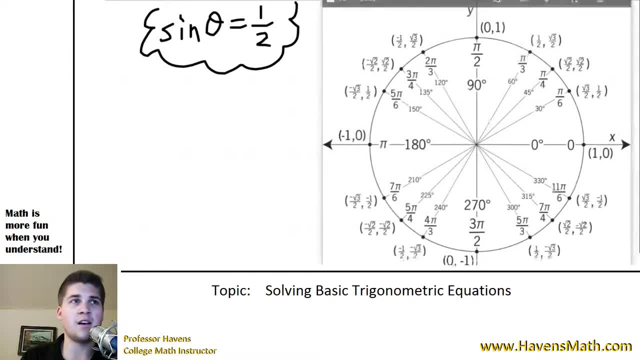 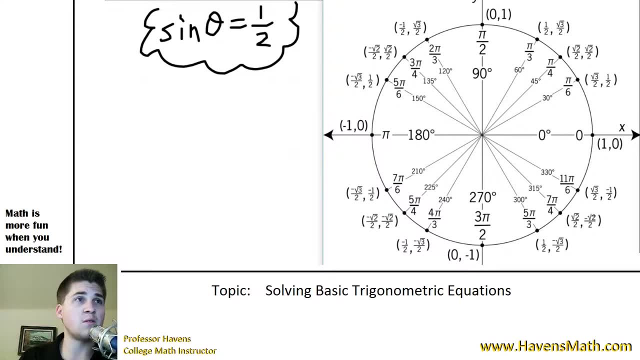 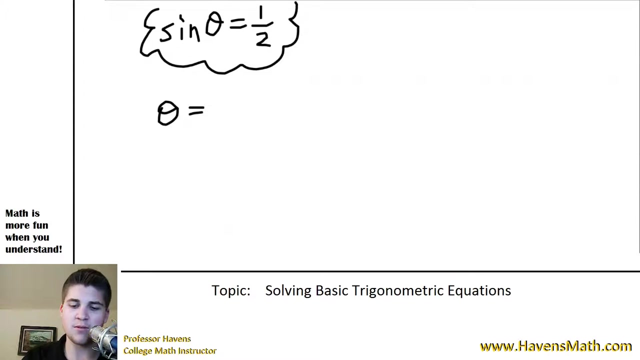 Remember that sine is defined to be the y-coordinate of our unit circle, different positions. So if we're looking for which angles would evaluate to be one half, we'd be looking on our unit circle for the y-coordinates of the particular points that would be one half. And if we look at that, we see that there's actually two positions on the unit circle that are one half. So right here, y-value is one half at the theta value of pi over six or 30 degrees, depending on. Which mode you're talking about, but we're going to, let's stick with radians for the time being, pi over six, and there's a secondary value, which on the unit circle, which would also have a sign of one half, which remember for your signs is going to be reflected about the y-axis. But if we take this angle and go directly across to the horizontal line, we see that the sign over here is also one half, and that would be what I call the secondary solution to this equation on the unit circle. So essentially. How we solve this one in particular is, well, we just look for where, where y is one half, because sign is the y-coordinate on the unit circle, and we see there's two pi over six and five pi over six. So we get that theta is equal to pi over six, and theta is equal to five pi over six. 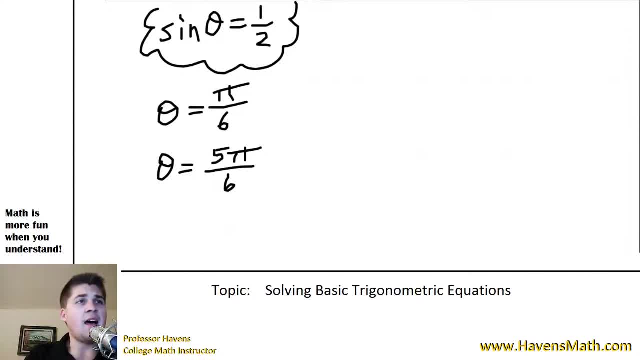 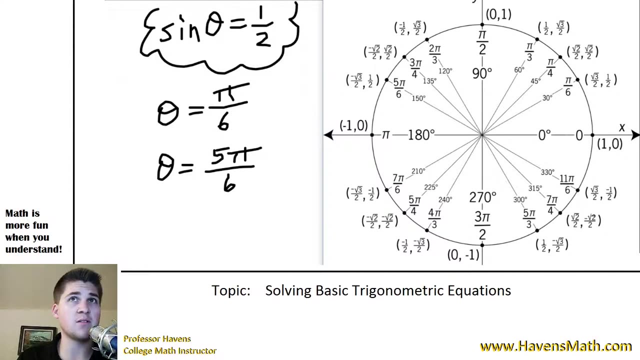 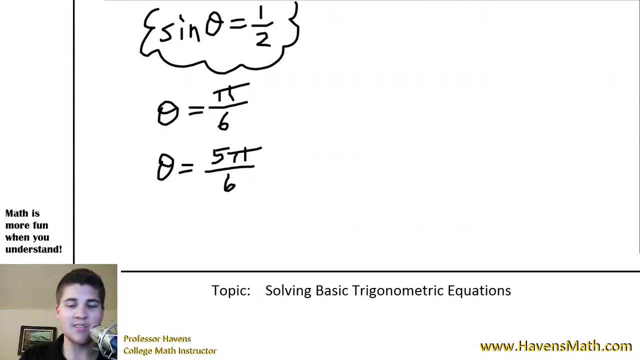 And so now these are just two particular solutions. Actually, this equation has an infinite number of solutions, because as you should be hopefully aware. Every, every position on the unit circle is, is repeated every, every two pi based on the periodic nature of the unit circle. So, you know, as we, as we work our way around, we have all these angles, but we can keep going and going and going in further, you know, in circles. And there are numerous different, what we call coterminal angles with the position, in this case, pi over six, or 30 degrees would be the same angle as if we went around again or added another 360 degrees to wind up at, in this case, 390 degrees. Or. If we added two pi to find the coterminal pi over six, it would be, uh, 12, adding 12 pi over six or, uh, pi over six plus 12 pi over six would make 13 pi over six. But essentially, um, my point is that, um, these solutions are just the two particular solutions to this equation on the unit circle. So while these are good, these are just two solutions. 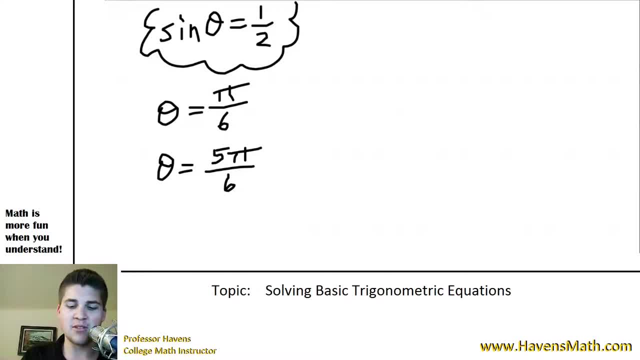 And so, um, a lot of times what you could be asked in these type of equations is solve all values in the interval zero to two pi. And essentially what this is saying is you want to find all, all the solutions on the unit circle. So if, if we're looking for all the solutions in the, uh, in the interval zero to two pi, we'd look for all the solutions on the unit circle, which there would just be two, uh, in this case, these two. However, sometimes you might be asked to find all of them instead. So, um, how we do that, how we add all those other repetitive angles, basically the repeated angles of these, these two particular values would be by adding two pi. Uh, as many times as we want, that would find all the cotermal values. We're adding two pi k. So as we, as we discussed in class, when you add plus two pi k, that will generalize it and find every solution. Remember where k is just a value, um, any, any integer value. 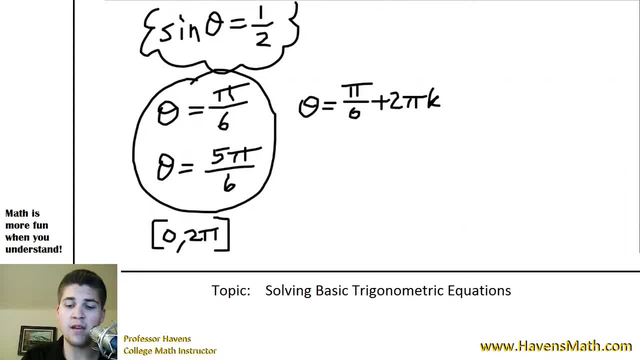 So one, two, five, a hundred, negative one, anything you want. So essentially if we, if we do this, we add, we look at those two values on the unit circle and write plus two. Two pi k, what this is, what this is essentially meaning is that, uh, we could use any of these two original angles plus any, uh, angle that is essentially the same when evaluated through the sine function, which would be all of these values as well. So these would be all solutions to the trigonometric equation as well. 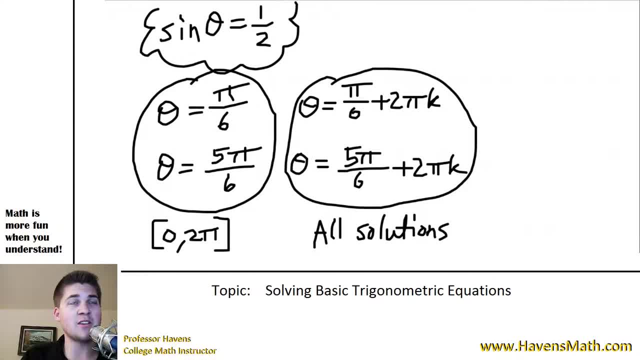 And so as some of you, uh, are aware, you could also solve an equation another way by using an inverse trigonometric function. Uh, you know, like if we're trying to solve just particular theta directly with our, our equation, if we start with sine of theta is equal to one half, and we take the arc sine of both sides. So we use the arc sine of the left-hand side would give us the arc sine of sine of theta. And we take the arc sine of the right-hand side as well. 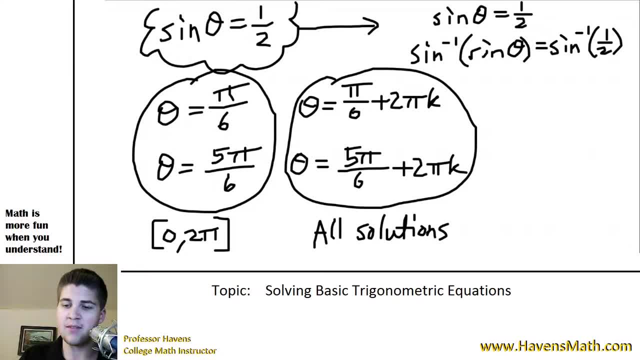 And due to the cancellation property, we'd say that the sine inverse and the sine cancel each other out, which leaves us with theta is equal to the arc sine. 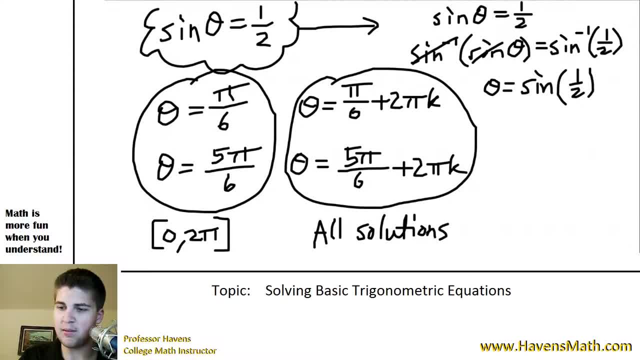 So that's one half. Oops, I forgot my negative one. 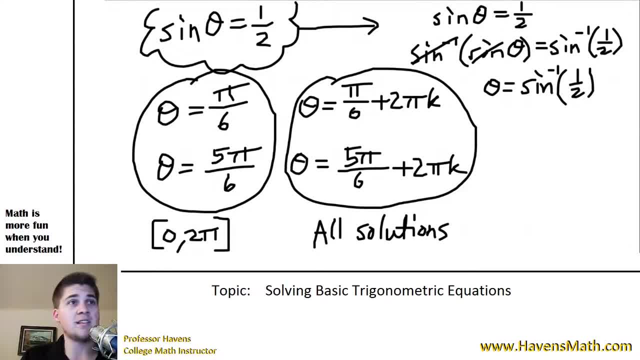 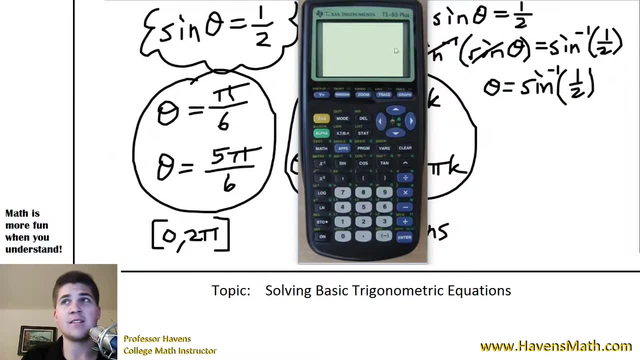 And, uh, essentially we could also use a calculator because calculators have inverse sine functions to solve for these values as well. Um, uh, but if we do use a calculator, we gotta be able to interpret that, that answer. So in this case, let's pull up, pull up my calculator here and go ahead and type this in. So, um, if we go ahead and type in the arc sine of one half, 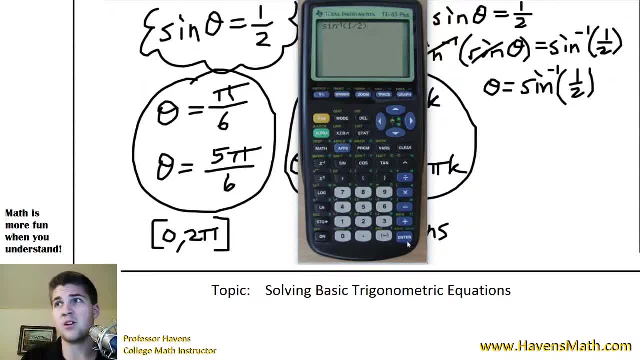 what we will get should hopefully be the same angle, which if we type this in, we get, well, this is some really strange answer, point five, two, three, yada, yada. 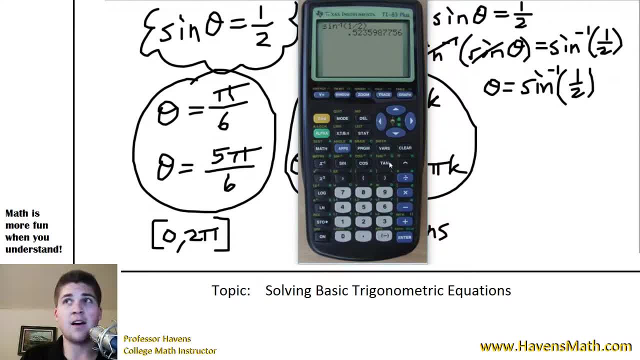 Um, which is actually the same if we look at it as, uh, our first solution over here, pi over six. 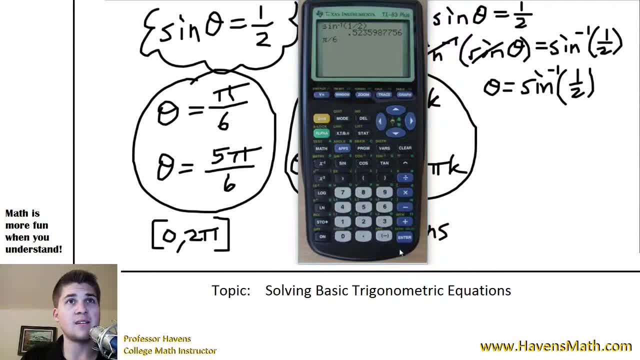 So notice that pi over six is that same value. 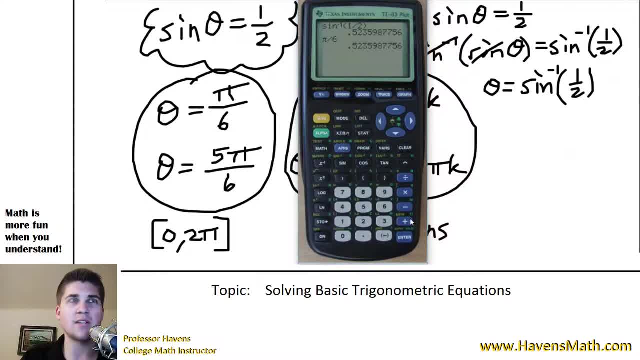 But basically our calculator gives us an approximation of the exact answer we already found, pi over six in radians. Um, so what, what, another, what we're going to do is we're going to go ahead and type this in. So we're going to go ahead and type this in. So we're going to go ahead and type this in. 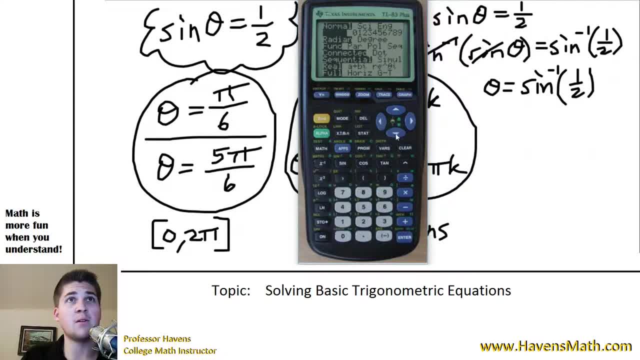 Another way, a thing that can be helpful to do on your calculator is switch it to degree mode, um, which will tell you the answer in degrees. And this will give you kind of a more exact positioning of your, uh, of your inverse function. 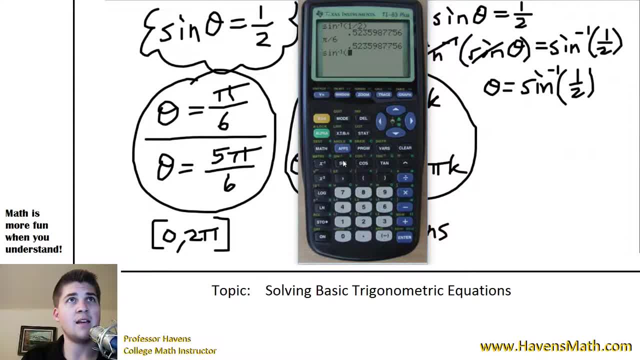 So if I go back and type in the sine inverse of one half now, um, what I would get would be 30 degrees, which again is that same position. 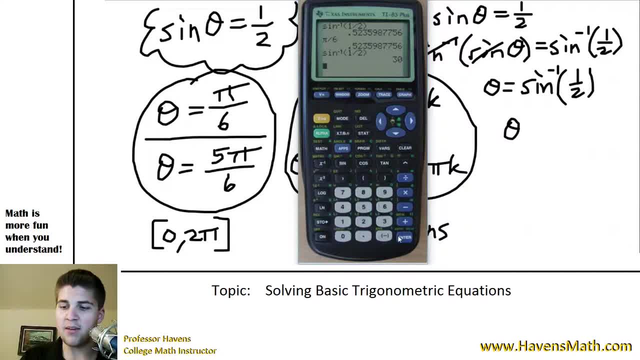 So, uh, essentially, uh, we would get that theta if we're in, if we're in radian mode, it'd be pi over six, which is, is indeed equal to 30 degrees, uh, in degree mode. 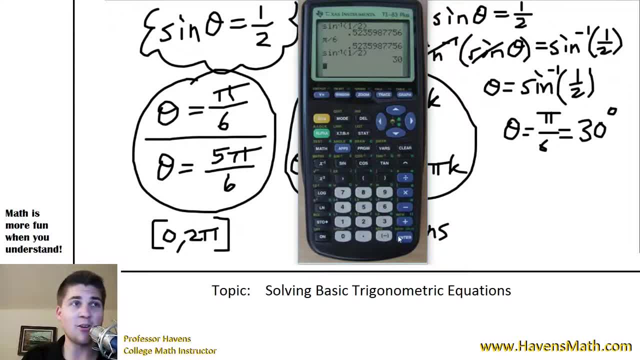 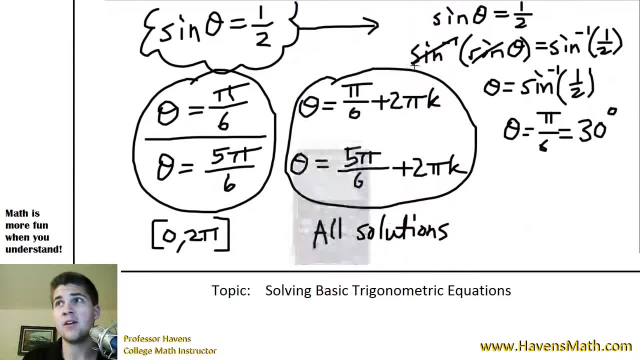 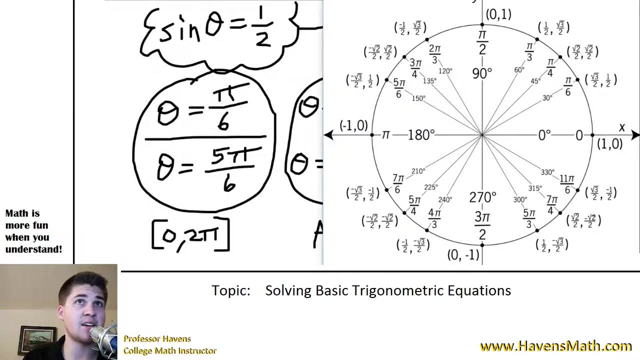 And so, uh, what I was saying earlier, sometimes you might be asked to solve your equation, um, you know, one way or another. Uh, so you could be asked to solve it in the interval zero to two pi, or you could be asked to solve it for every value in radian mode. Or sometimes you could be asked to solve it for all values from zero to 360 degrees, basically, uh, also on the unit circle, but in degree mode. And then basically our answer, and if we're asked to solve it in this form, would be 30 degrees, uh, so, but, uh, the limitation of the inverse function is that it only gives us one value. The secondary solution is when we have to find, so in this case, again, it's going to be the same angle, uh, going back to the unit circle. If we look at that first angle that the inverse function gives us, it's always for sine, the secondary answer is directly across. 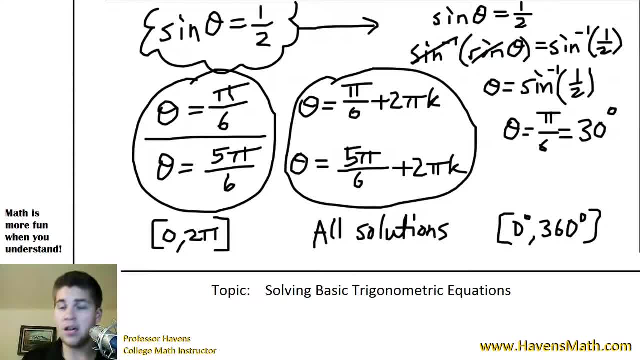 So in this case, 30, our secondary solution would be 150 as well. And so we would get another solution. And so we would also have the same value. We would have the same solutions if we're, if we're using degree mode as well, and kind of, so here's my point. You can use a calculator to calculate these as well, uh, if, if it's a non-unit circle value. So as you can see, there's a lot that goes into solving a very simple trigonometric equation. But basically, um, you can use a calculator, you can use the unit circle. Uh, if it says, say your equation was sine theta is equal to 0.6 or some value that's not on the unit circle, then, uh, it's, it's a little bit simpler to directly, go to the calculator, um, to solve those. And that's actually going towards our next example. 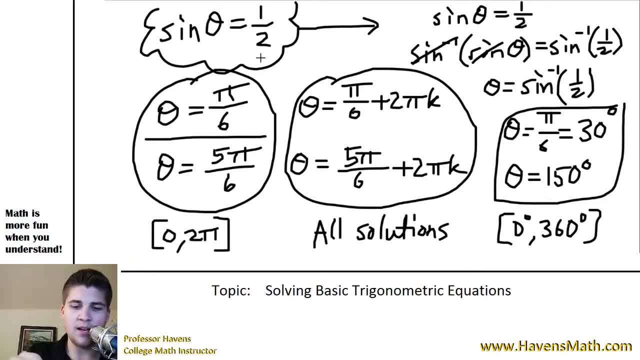 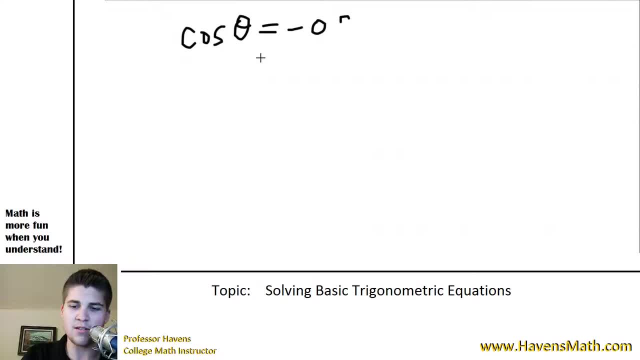 So the next example we're going to look at would be, let's say we have, uh, cosine of theta is equal to negative 0 point, let's just say 0.2. 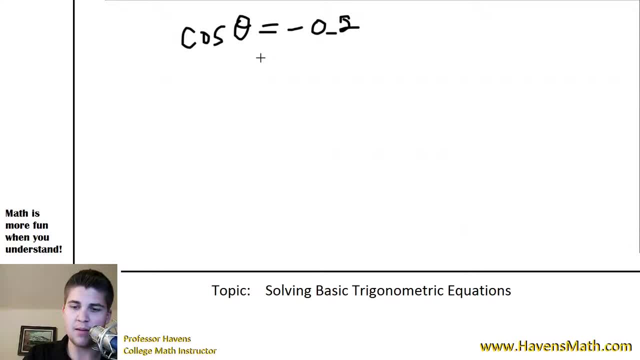 So, sorry, let me fix that, um, tablet's a little bit finicky. Okay, so 0.2. 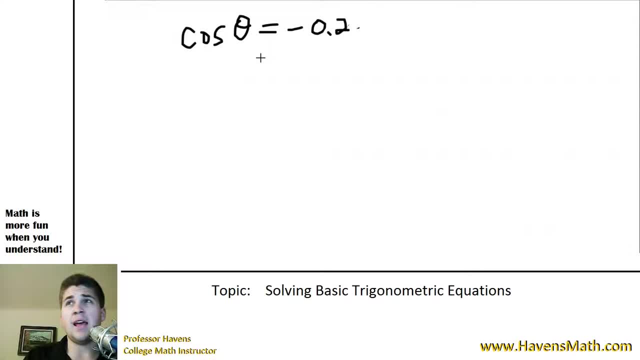 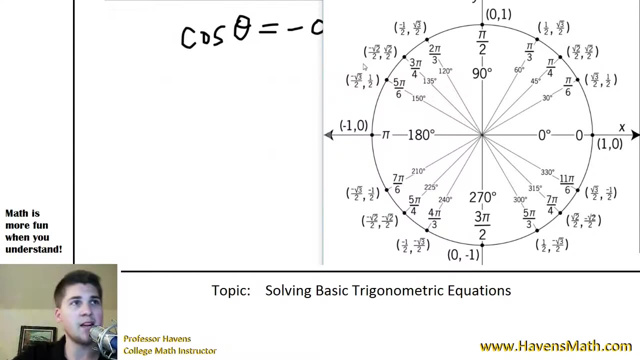 And so if we want to solve this as well. So again, if, if we're looking for where cosine is negative 0.2, um, basically it, what we would be looking for on the unit circle, well, where is our x coordinate? Because remember, cosine is defined to be the x coordinate on the unit circle. 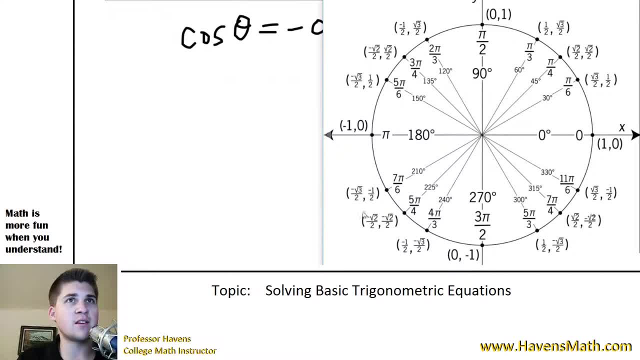 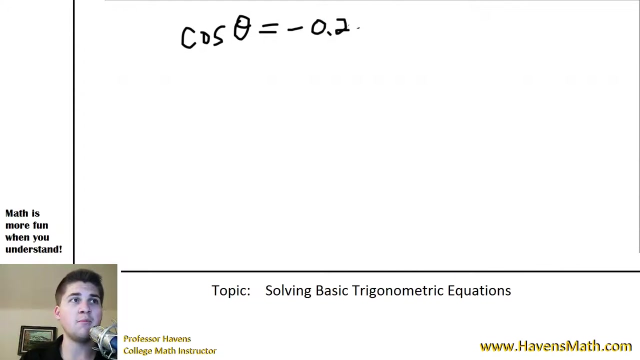 Where is cosine negative 2? And, you know, with initial inspection, you know, on the, our unit circle values, uh, none of those values for x is ever negative 0.2. And where 0.2 would be? Well, it, remember the unit circle's, uh, a distance 1 away. It would be somewhere over here, a point that we do not have negative 0.2 would correspond to, uh, one of these two values over here. If you drew a vertical line through point, negative 0.2, that would give us those two points on the unit circle where, um, cosine would evaluate to be negative 0.2. Again, since this is not a solved point, it, uh, it's not a special angle, um, we would actually need to use a calculator in this case. Okay. To solve this. 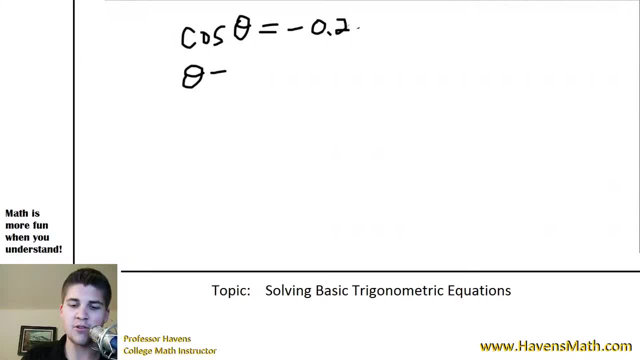 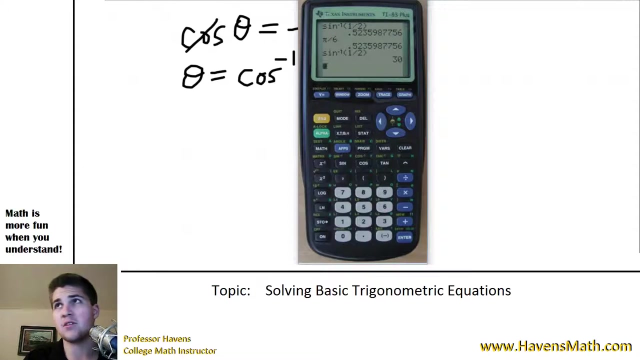 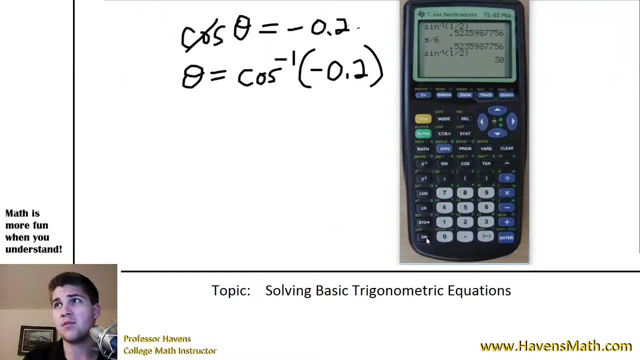 So again, similar, similarly, we would take the cosine inverse of both sides of this equation, which would give us cosine inverse of negative 0.2. Again, I, my trick was to just move it across the equation as an inverse, but really what I did is I used, I took the cosine inverse of both the left-hand side and the right-hand side, which cross, canceled out that cosine on the left side, moved it over. Kind of like when you're, when you have x plus 5 and you want, equal to 7 and you want to solve. You subtract 5, you use the inverse of adding, subtracting, so if you're trying to get rid of the cosine function, you cannot divide by cosine, that doesn't work, because it's a function, um, you can't just divide it away, it doesn't make sense for functions, uh, but the inverse function will cancel it out. So anyways, we get theta is cosine inverse of negative 0.2, again, can't, can't evaluate this without a calculator, so let's go ahead and do this on our TI-83, so we'd have the cosine inverse of negative 0.2. Again, can't, can't evaluate this without a calculator, so let's go ahead and do this on our TI-83. We'd have the cosine inverse of negative 0.2, and that gives us a value 101.53, and if you remember, I'm in degree mode, so basically this theta value is 101.54 if we round to, say, the nearest hundredth place. Again, the decimal place is not incredibly important, usually. 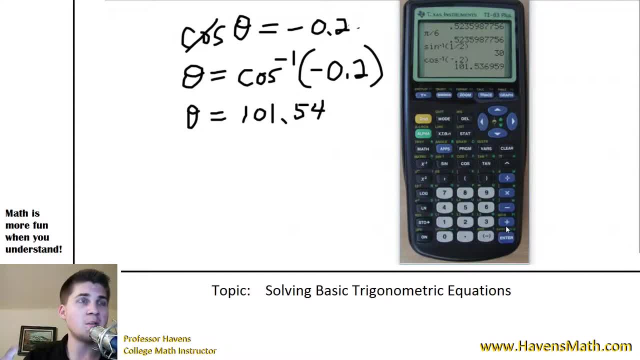 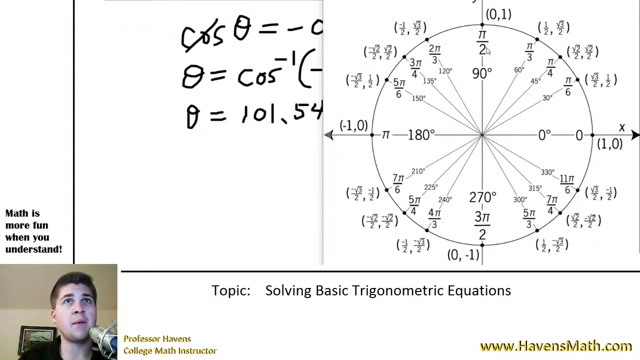 Um, unless you're solving a triangle or something where too much rounding can cause problems, but in this case, um, we get our theta value, it's about 101.54 degrees, and again, what I mentioned before, kind of like with the last example, trigonometric equations usually, well, they always have infinite solutions, well, assuming it has a solution, but, uh, on the unit circle, there's usually two. So, um, our inverse function gives us one, the secondary solution in this case, if we look at that angle, 101 degrees, uh, would be... Uh, a little bit past 90, because 0, 30, 45, 60, 90, it'd be somewhere up over here, uh, and so that cosine would have, again, the x value up there would be negative 0.2. So the secondary solution with cosine is not over here, like with sine, it's actually directly down here. So the secondary solution where cosine would be negative 2, negative 0.2, uh, would be down across the unit circle, reflected about the x-axis. And so then, kind of the idea... The problem with this is we've got to figure out, well, how do we get to this angle, how do we know what this one is? We know that this one up here is 101 degrees, how do we find this one? What's nice about cosine in this case, the first solution is a positive 101 degrees, the next... 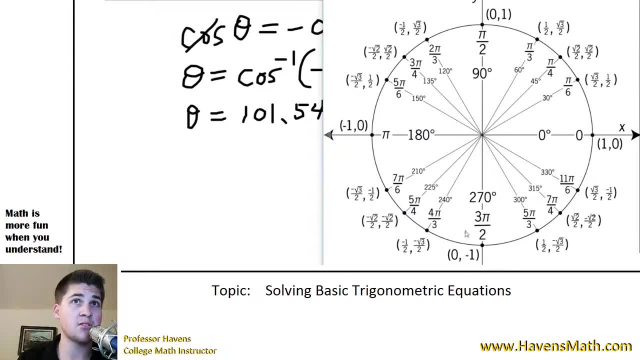 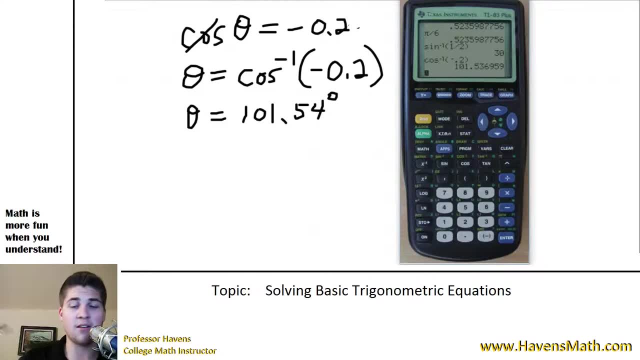 The other one's going to be actually symmetric directly in the same position down here, it would actually be negative 101 degrees, the same answer but negative. So the secondary value would actually be theta is equal to negative 101.4. Uh, 0.54 degrees, uh, and that would give us that other position, um, so, um, again, these are two solutions, but a lot of times we're going to be asked to solve, say you're asked to solve in the interval 0 to 2 pi, or 0 to 360, or whatever, 0 degrees to 360 degrees, or whatever other intervals you're asked to solve them in. Um, so these two answers are good, but, um, the second answer, the negative 101.54 degrees is not in... Either of these intervals, so, well, how do we find it? Well, uh, we could simply find the coterminal angle by adding either 2 pi or 360 degrees, uh, depending on what mode we're in. In this case, we're in degree mode. That angle is the same if we rotate one full circle around, we can get back to the same position. Basically, if we add 360 to that, we would get the same angle, um, and, uh, again, we call it coterminal, but in this case, we can add 360 to that. 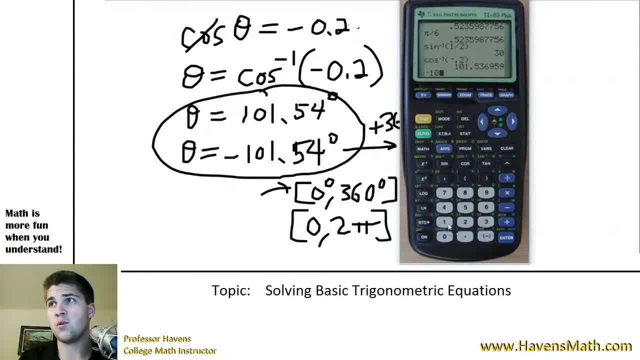 So let's go ahead and take our, um... Let's take negative 101.54 and add 360 to that, and this will, will figure out what that angle would be as a positive angle. 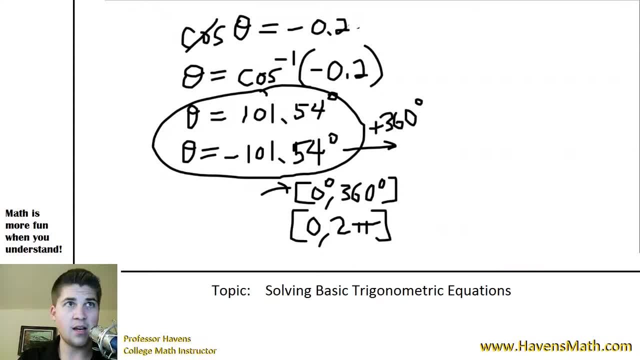 258.46 would be our solution, and notice that, um, this angle here is actually within the interval, so if we're, you know, in those pesky questions where they ask you to solve it between 0 to 360, uh, that can help us find our two solutions. So, at the end of the day... 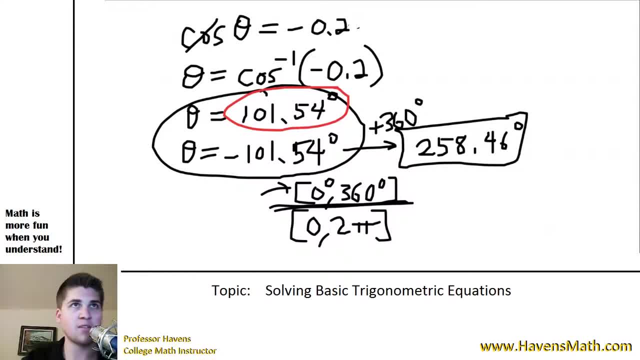 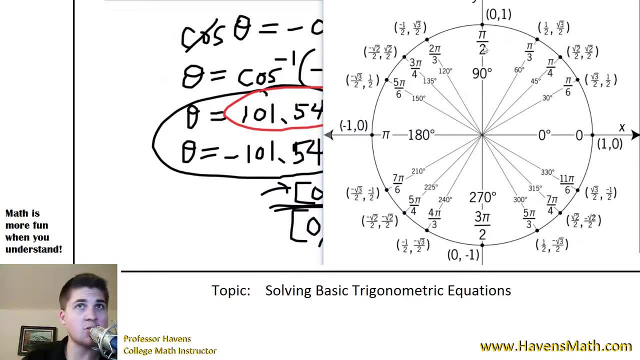 Two solutions in that interval would be the first solution given by the inverse, and the second, we had to take that away from 360 to find it, essentially find the same angle reflected downwards. Or if I kind of put these together now on the unit circle, our first solution was 101 degrees, our second solution was down here at 258 degrees, so as we move our way around, 240, you know, 180, 210, 225, 240, 256 would be down here. Again, that would have the same cosine, negative 0.2. They would have the same x-coordinate at those two positions. So that's how I knew to do that, to find those, and that's what's tricky about it. 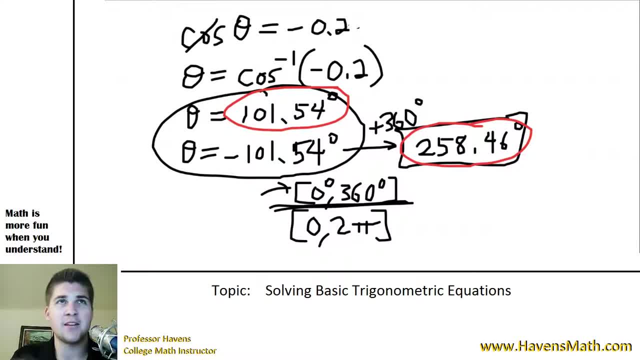 You've got to really understand your trigonometric functions to understand how to find those, and then those would give us our two solutions in that interval. And then if we wanted to find, uh, if we wanted to say all of them, you could add 360 degrees over and over again to find coterminal, so, or you could convert them to radian mode if you just set your calculator in radian mode instead of doing it in degree mode like I did there. We would get an approximation for those answers, it wouldn't be, uh, like pi over whatever, it would be, um, probably some decimal, like 101 degrees is something around 1 point, uh, 1.7, 1.8 radians, something like that, so it's going to be a dec, these are both, will both be different, uh, decimal numbers. Remember, you can always take your degree answer, multiply by pi, and divide by 180 to convert those to radians after, if, if you like that method as well, uh, to solve those, but at the end of the day, that equation, 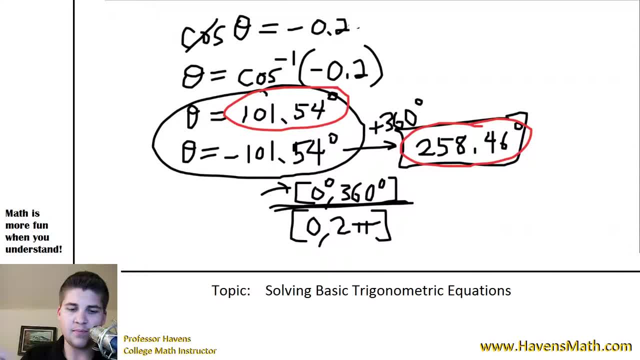 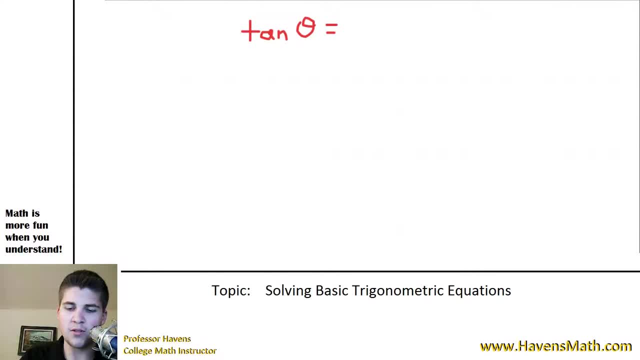 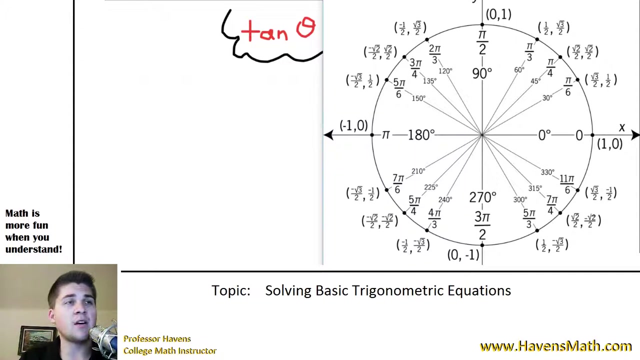 So let's do one last example, let's try to do a tangent, uh, of something, so let's say we had the equation, um, tangent of theta is equal to rad 3, and so, um, in this case, this, we, this is actually a position on the unit circle, um, and the reason I know that is because root 3 is a, is one of those numbers that's very common on the unit circle, but remember, tangent, uh, tangent is the ratio between y and x, if we look at the definition, so, essentially, we're looking for where on the unit circle is our ratio between y and x, rad 3, or rad 3 to 1, a ratio of root 3 to 1. Um, so if, uh, again, putting back up the unit circle, um, where, uh, we're looking for a y value of root 3 and an x value of 1, which actually occurs in two positions, um, so at pi over 3, right up here, uh, our y to x ratio is root 3 over 2 to 1 half, and so the tangent here is going to be this, divided by this, which is going to give, uh, root 3 over 2 divided by 1 half, and as you guys hopefully have seen by now, that's going to just be root 3 divided by 1, or root 3, and the secondary for tangent is actually directly across the unit circle down here, at this position as well, tangent would be a ratio of root 3 over 2 to 1. 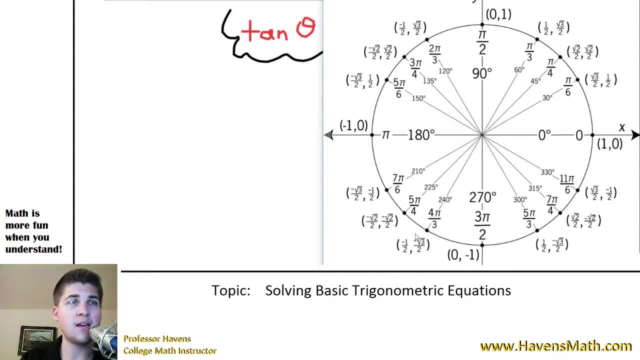 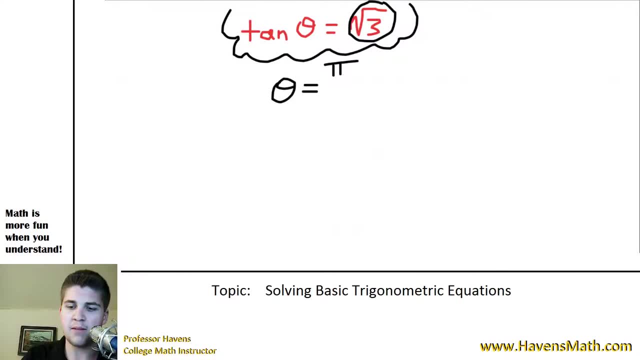 Right, so, I'm just going to, uh, say that we're going to get ridiculous answer here, which is, well, um, we can't get 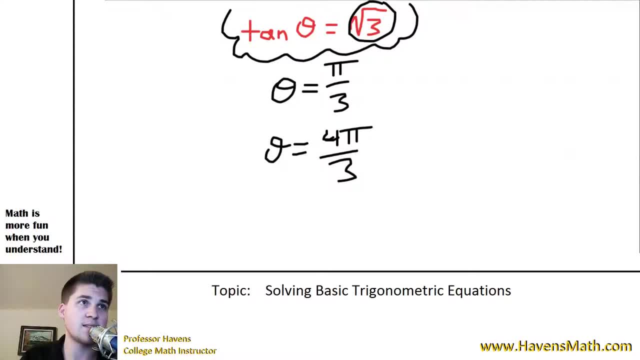 Um, this is so interesting, because, and we'll come back to this in white in a moment, but we know that the solution for negative 1 half or negative 1 half Nergative to negative would make positive. And so, pi over three and since tangent the secondary solution is always a half a period away plus pi away you can just add pi k and this would generalize all of our solutions for our tangent despite the interval but again these would be the two pi over three and four pi over three would be the two that are in the interval zero to two pi but if we wanted to extend those to all solutions we would just add pi k to do that uh please let me know if you have any questions in the comments have a good rest of your day and see you around